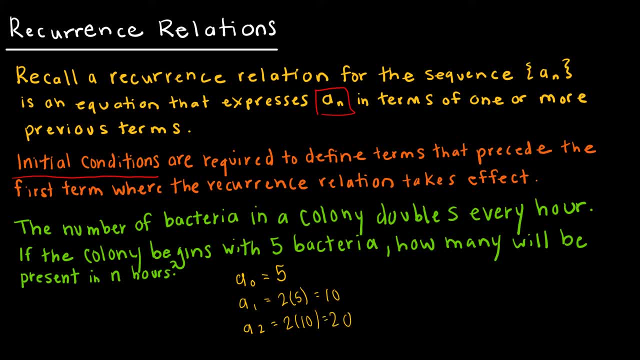 is 20.. And really I don't care about those values. What I'm looking for is how am I going to express this in terms of whatever happened before? So if I were to write my recurrence relation, I know that when I found A1, I was taking 2 times A0. And when I found A2, I was. 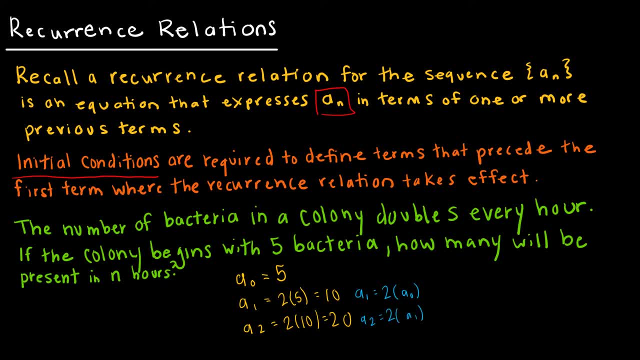 taking 2 times A1.. And so my recurrence relation. my answer would be that I start by saying that A0 will be 5. And then anything after that is going to be taking 2 times the previous value. So A sub N is 2 times A to the N. 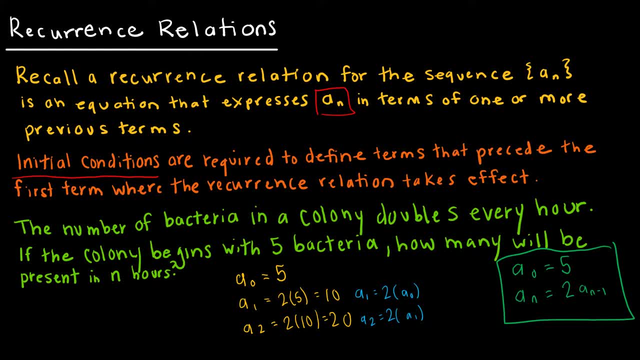 And again, it's best to use N here instead of using A to the N plus 1.. That can get a little bit confusing, So this would be my solution for writing it as a recurrence relation. So let's take a look at an example. We are looking at the same example we just looked at. 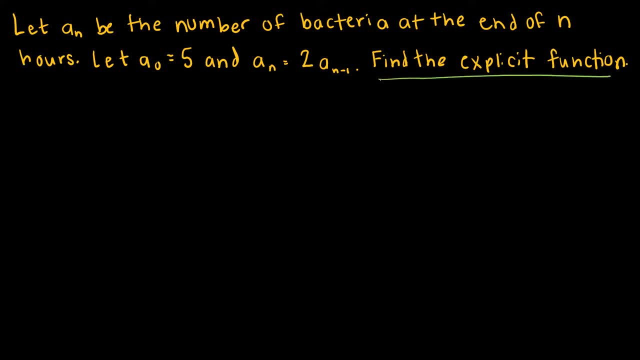 but what I want to do is I want to write it as an explicit function instead. So this is the recurrence relation And I'm going to write it as a recurrence relation And I'm going to write the recurrence relation And I'm going to write the recurrence relation And I'm going to write the. 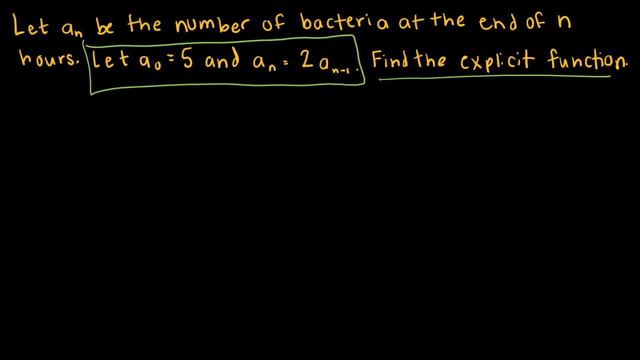 recurrence relation that we had come up with previously. Remember, it has two parts, That's, the initial value and the recurrence relation. Now I want to find an explicit function which means, instead of relying each time on what value did I have before, which is what happens in a recurrence- 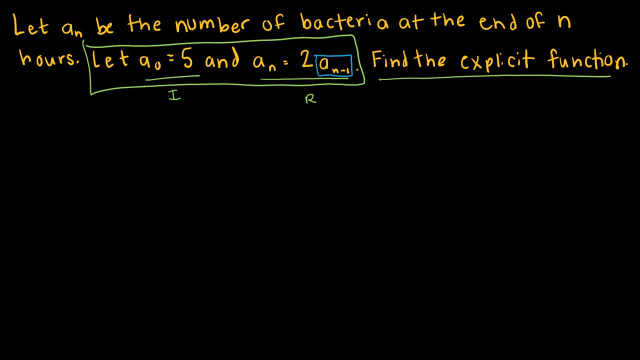 relation. I want to write it so that all I have to do is input N somewhere and find a solution. So let's take a look at the process I might go through in order to do that. Remember that A0 is 5.. My first value is 5. A1, according to my recurrence relation. 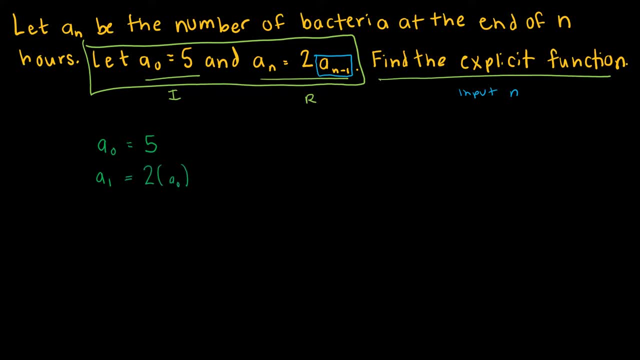 says, take 2 times A0. And 2 times A0 would be 2 times 5. And I could write that as 10, but I'm just going to leave it as 2 times 5.. A2 would be 2 times A1.. And remember, A1 was 2 times 5.. So I could really write that as 2. 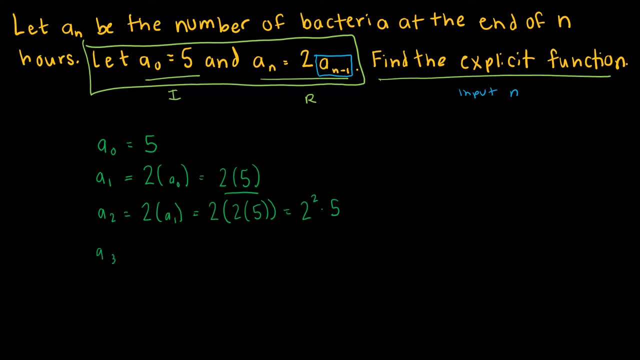 squared times 5.. And then A3 would be 2 A2s, And that means 2 of all of this, So 2 times 2 times 5.. Or 2 to the third times 5.. So we can see what's happening here. This was really 2 to the 0 times. 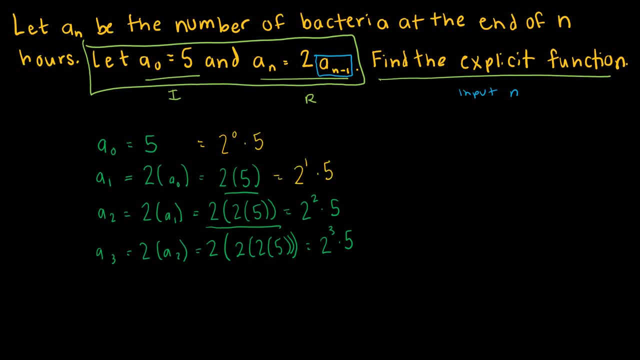 5.. And this was 2 to the first times 5.. And so, if I keep going, I can say that the nth term, any term that I want, would be 2 to the n times 5.. So I found it just by looking for the pattern. 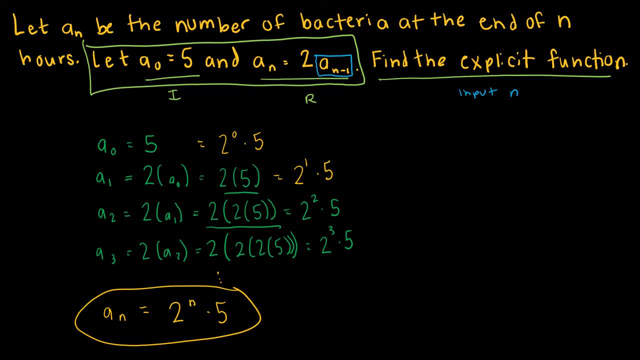 We call that basically an iterative sequence, So we're looking at each term and how it relates to the term before it. So now, if I wanted to find A3, which I had previously found to be 2, to the third times 5,, which would be 40. Instead of having to do that, 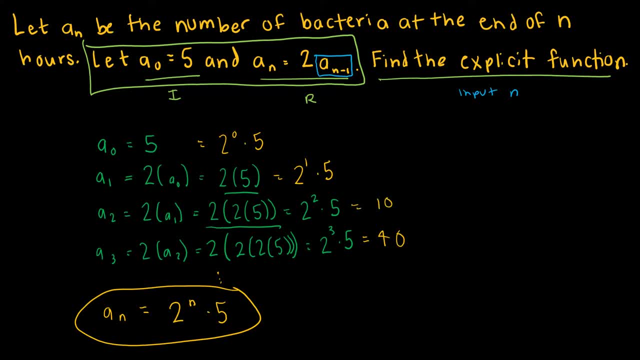 by finding that this was 10 and then taking it- I'm sorry, this was 20- and taking it times 2, and this was 10 and taking it times 2, and this was 5 and taking it instead. I can just say, hey, if I want A3, that's going to be 2 to the third times 5,. 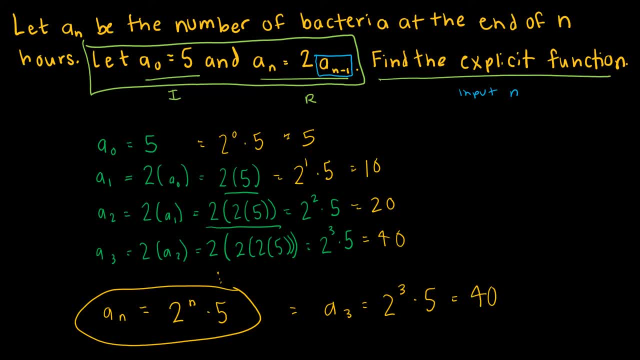 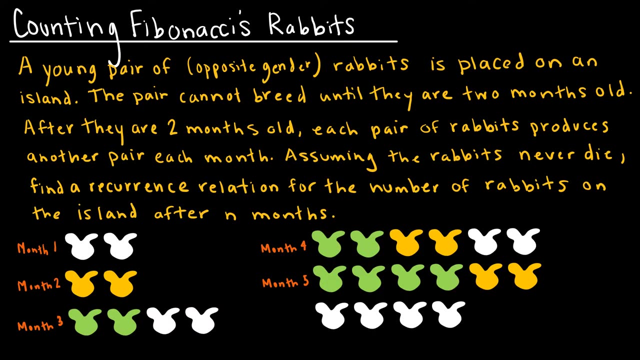 which is 40. And it's just a lot faster, Especially if I'm looking for something like A200. Then I would definitely not want to have to find all of the 199 terms that happened before. Now let's take a look at how the Fibonacci sequence came about. So, a young pair of 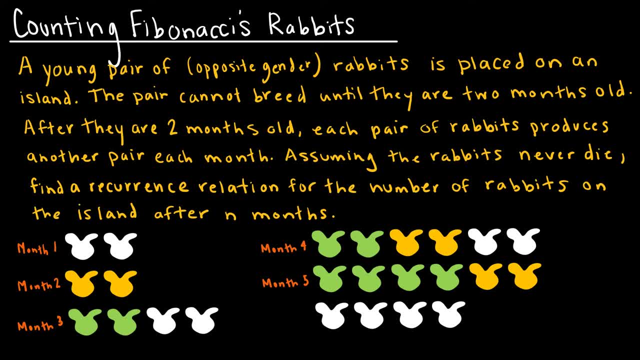 opposite gender rabbits is placed on an island. The pair cannot breed until they are two months old. After they are two months old, each pair of rabbits produces another pair each month. And let's assume, scarily enough, that the rabbits never die. We're going to find a recurrence. 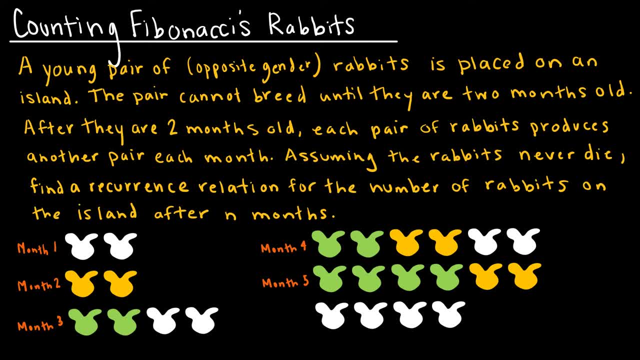 relation for the number of rabbits on the island after n months Now. we've already talked about the recurrence relation for Fibonacci numbers, but this is how it came about, So let's take a look. The first month we have my two rabbits. 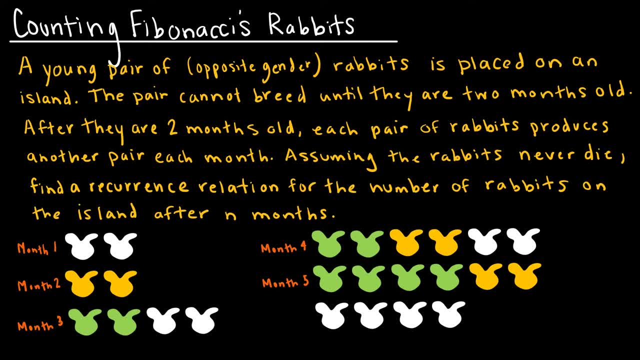 Male and female. we have a pair, And they're too young to be breeding. The next month, month two, they're now old enough to breed but have not yet reproduced. So then, month three, these two guys create two brand new rabbits. So I've got two. 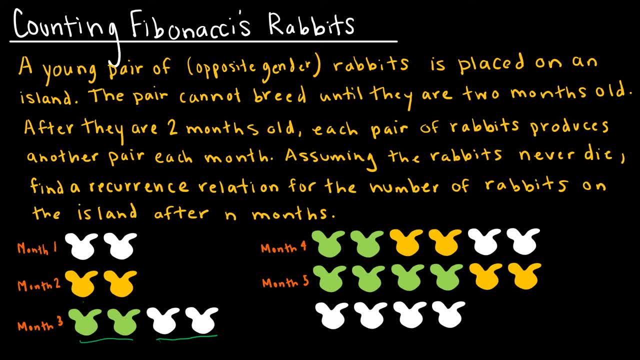 a pair that is ready to breed and a pair of brand new little babies The next month. these guys are still ready to breed. Their new little babies are a month old, so they're not. they're ready to breed for the next month. And then the green couple had another pair of babies. 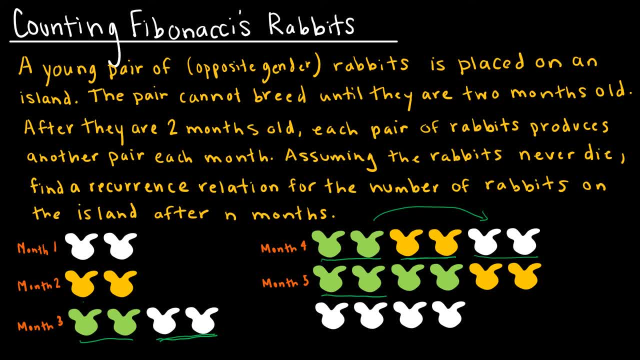 So my green couple stays green. These guys who were yellow, now are old enough to breed. Both my green pairs have had a pair of babies and these guys. they're now ready to breed. So this is kind of the pattern that we're going through. 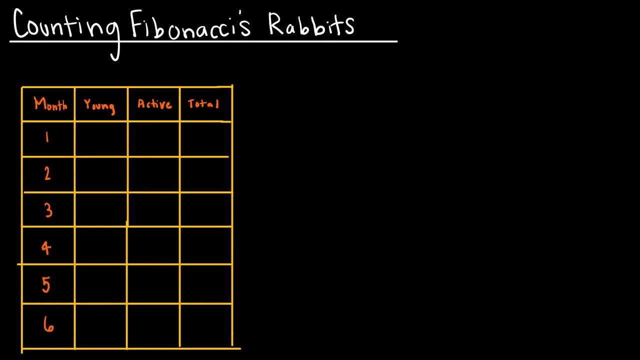 So let's take a look at how we might put this in a table form to maybe help us to make sense of what's going on. In the first month I have one young pair. They're not able to reproduce yet. I don't have any reproducing pairs, so I have just a total of one pair of rabbits. 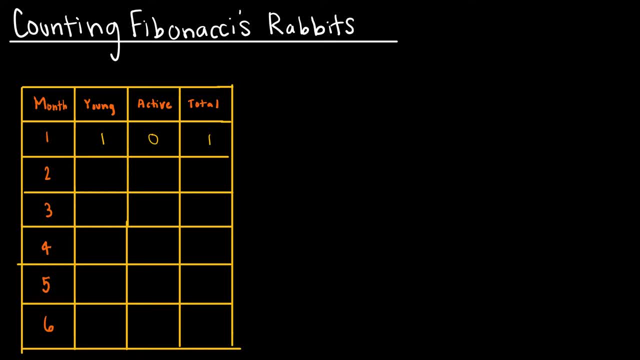 In the next month. my young pair is old enough now to reproduce, but hasn't yet reproduced, So any active rabbits will be. of course we're going to take that time, you know, or get another pair out of them. 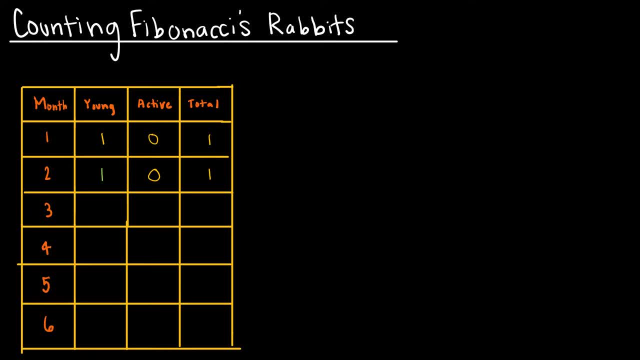 So right now I still just have one. Now, my young pair has now moved over here And because they've moved over there, they've had a baby. And so well, a pair of babies, I guess we would say. 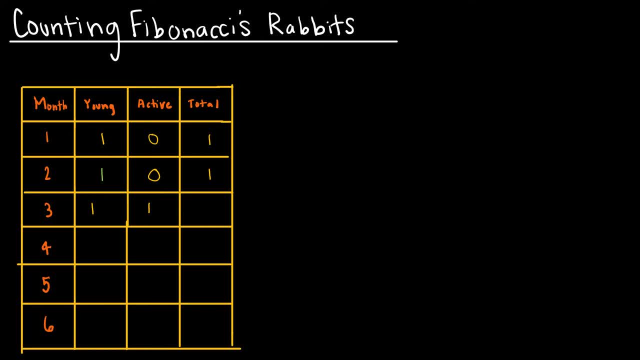 And so in month three I have my active pair and my young pair, and my young pair is not old enough to breed yet. So now I have two total pairs of rabbits. In the next month I still have my active pair, and my pair that was young before is now old enough to reproduce but has not yet reproduced. 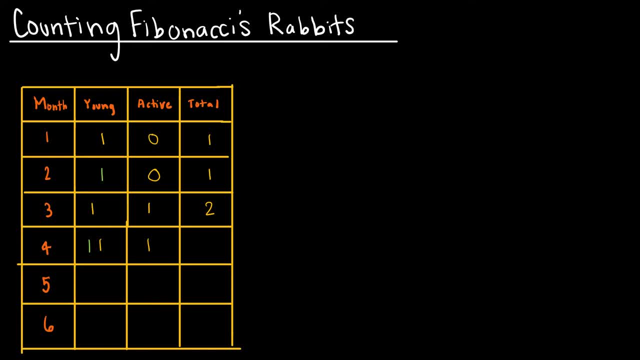 But my active pair has had another pair, So I have a total of three pairs of rabbits Again. this time my active pair is still active. the this pair of rabbits is now active as well, And they both reproduce a pair of rabbits. 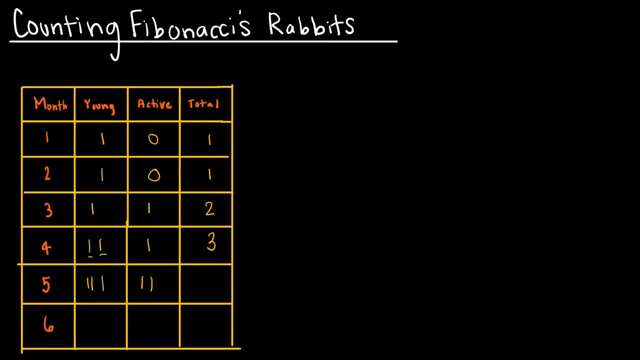 My non-reproducing pair is now ready to reproduce. My non-reproducing pair is now ready to reproduce on the next try. And so right now I have five pairs of rabbits. Then again, following that same pattern, I've got my two active pairs, plus my guy who's becoming active, my pair who's 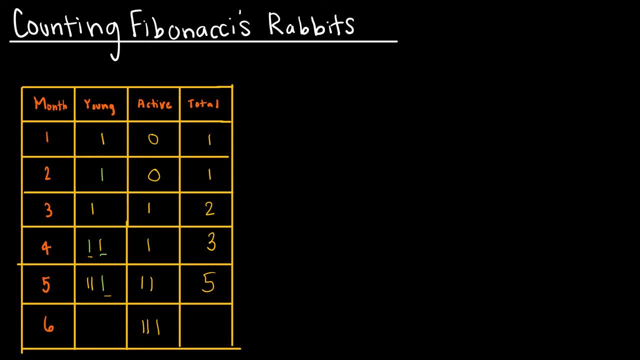 becoming active, And each of those pairs has a baby. In addition, I've got my two that were not ready to reproduce are now ready to reproduce, And so now I have eight. So here's sort of the way that this is set up, And before we look at it in terms of a recursive definition. 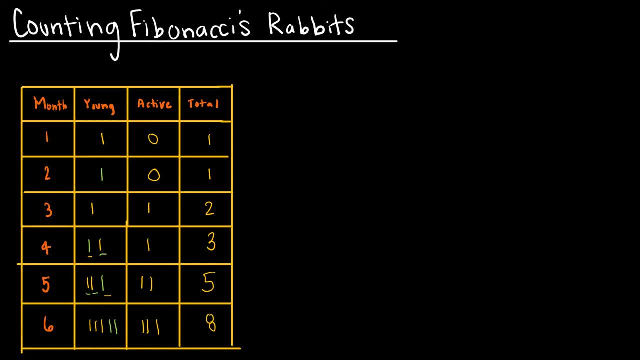 I want to just point out to you that this value matches this value, and this value matches this value, And we can see that that's going to be helpful to us as we're moving forward. So what I'm looking for is: how am I going to write this so that it makes sense? 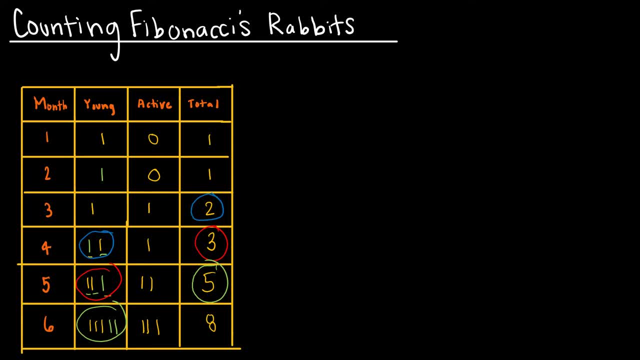 Well, really, what I'm looking at is I'm taking to find eight, I'm taking the number of pairs that I had before, And then I'm also adding the three, because those are going to be the couple that are old enough to reproduce. So what I'm looking at is: how am I going to write this? value, And I'm also adding the three because those are going to be the couple that are old enough to reproduce. So what I'm looking at is: how am I going to write this value? And I'm also adding the three, because those are going to be the couple. 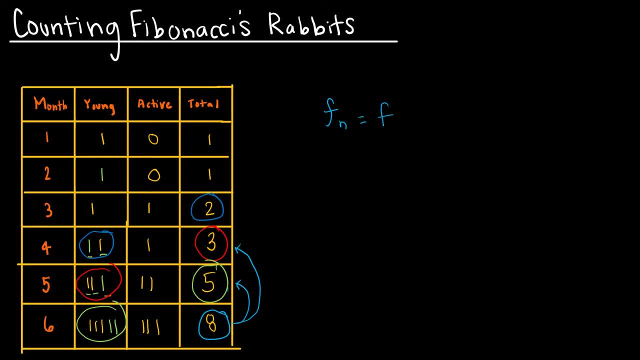 is to find the value. I'm taking the value before that plus the value before that. So I'm taking f of n or fn equals the two terms before that. Now, remember that it's only a recurrence relation or a recursive definition if it also includes the initial conditions. 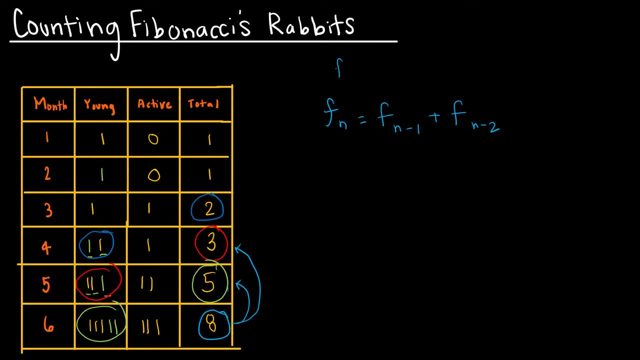 And of course, the initial conditions are that in the first month I have one pair of rabbits and in the second month I have one pair of rabbits. So this is the initial And then from here, this is where the recurrence relation takes effect. 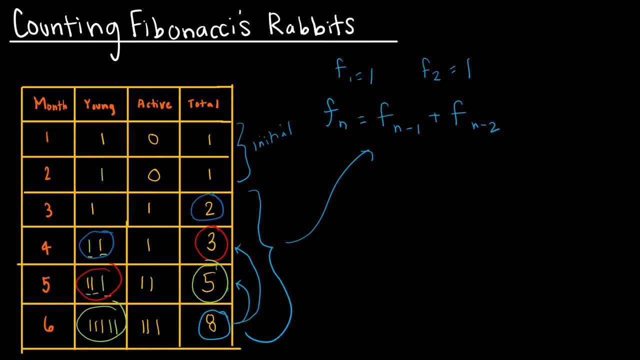 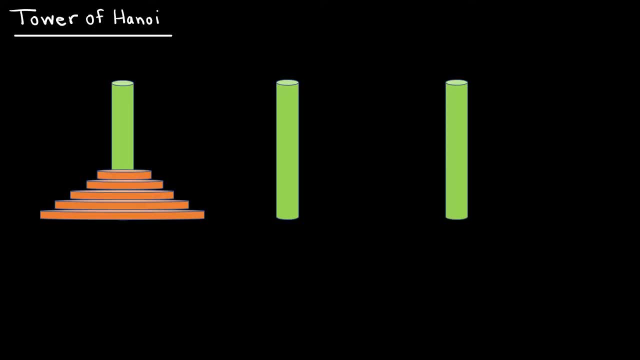 So now I can use that recurrence relation to determine, say, how many rabbits I'll have in month 10 or 20 or 100 or 1000.. Let's take a look at the Tower of Hanoi question And the Tower of. 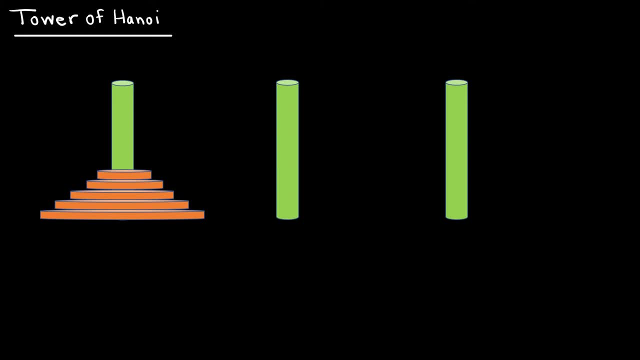 Hanoi is basically a popular puzzle that asks you to take disks and move them from where they are located. we'll just call this one over to two, And we want to move them to two so that they're in the same order that they are in now. However, I can only move one disk at a time And I can only 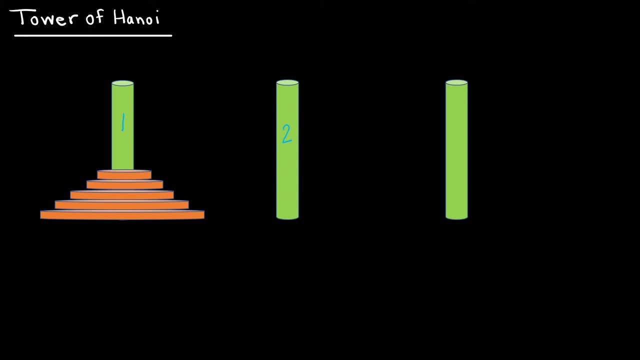 stack disks so that the larger one is on the bottom and the smaller one is on the top, which means I move this guy and then move the next one, and move the next one all over to three and then move them back. it's not going to work that way. So what I'm looking at here is to write this as a recurrence. 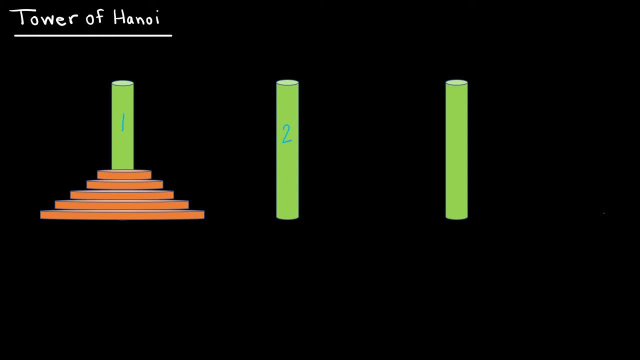 relation. So I'm not trying to find this explicitly yet. I just want to look at the recursive definition of how I would write this. So remember that a recursive definition starts with how many times would it take for, say, one disk. So for one disk, if I just had one guy, I would just have one move because that one. 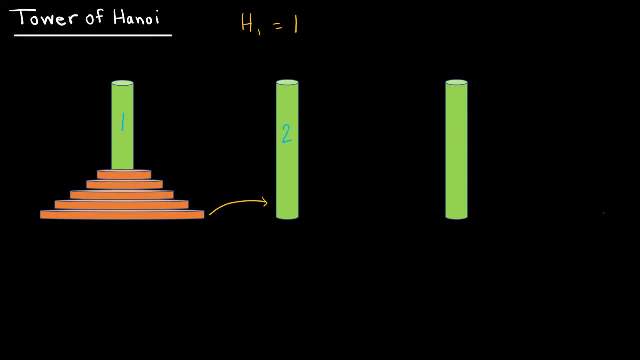 move would take the disk here and move it to tower two, which is where I want it. this is where we want them to all end up. So great. there's my initial condition. Now I want to find what's the recursive definition, And remember that I'm not looking for a specific number, I'm just saying in. 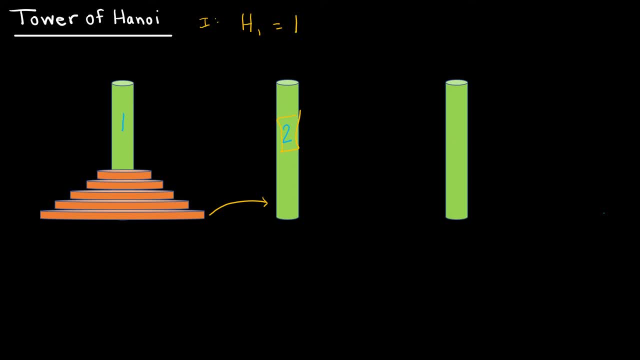 terms of what, In terms of some value before. So what I know is that this set would be n minus one discs, because I start with n discs And what I need to do is take these n minus one discs and move them over here to three, so that I can get to this last disk, to move it over to two. 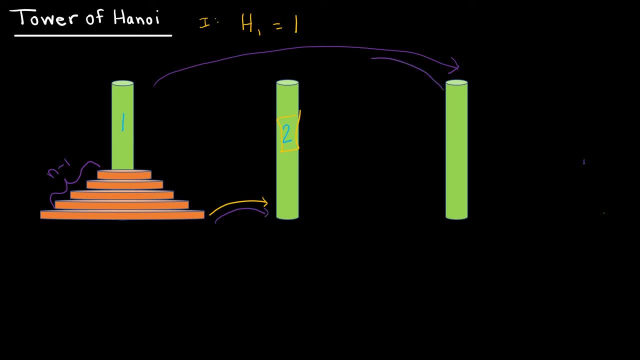 and then I have to take all of those discs and move them back to two. Now again, I'm not saying how many moves that will take, I'm just going to write this recursively. So my recursive part of the definition is saying: to find the number of total moves I'm going to take two times the 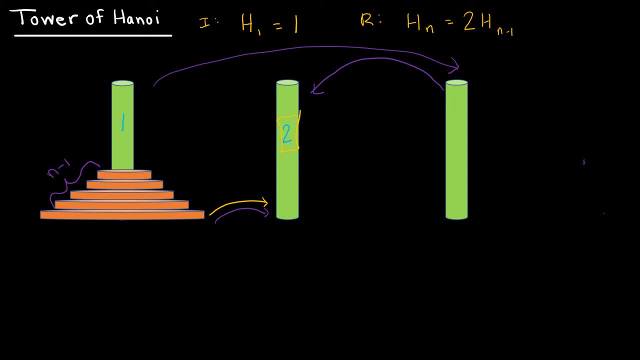 number of moves it would take to do n minus one discs, and then I'm going to add one so that I can get the bottom disc where I want it to go. So this is my recursive definition, and you might think, well, that's not super helpful and it's not yet because, again, this doesn't help me unless 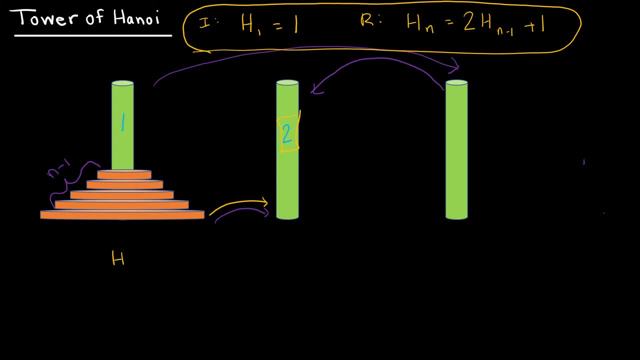 I want to take the time to say: hey, if I do this with just one disc, then it's one move, And if I do this with two discs, then I have to move the smallest disc over to three, so that's one move. 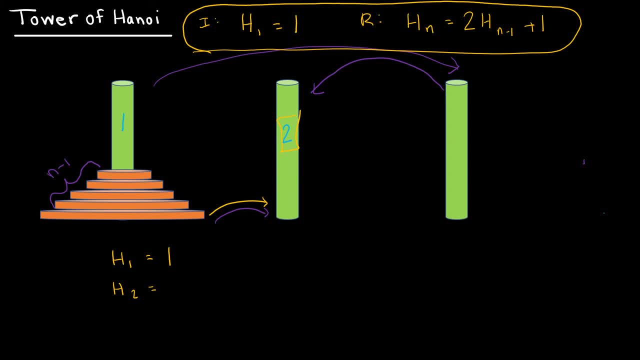 and then the bottom disc to two, so that's another move- And then the smallest disc back on top to two, which is three total moves. And so if I wanted to keep this going for three, for four, for five, and look for a pattern that way, I could. but 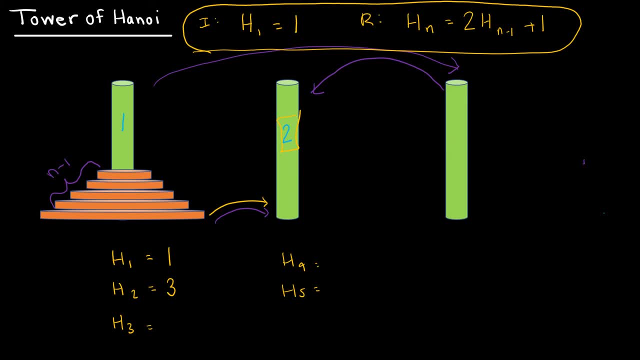 instead I sort of went the opposite direction and said: this is how many it would take to move n minus one discs, and that's all I need for a recursive definition. So again, that's not super helpful, because what I wrote was: I'm going to take the number of discs and then I'm going to 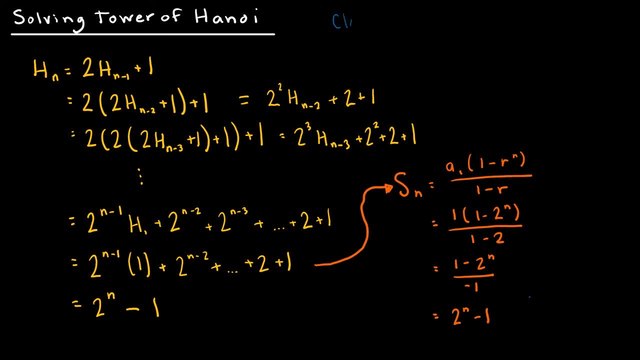 use this, And I'm going to take the number of discs, and then I'm going to take the number of discs. So that's really what I'm going to be doing here. What I want more than anything is a closed form or explicit definition, And that's what we're going to do now. Now, I wrote it out ahead of. 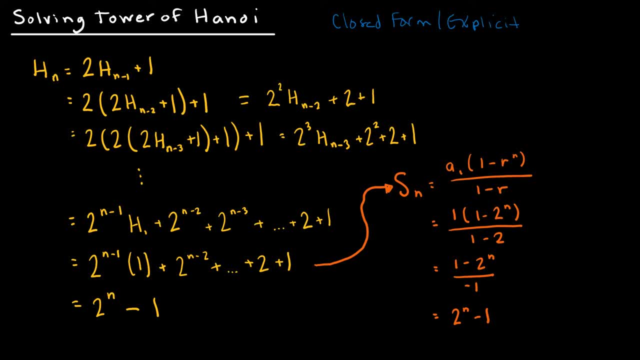 time, because I am prone to making mistakes when I'm trying to write things that are complicated and speak at the same time. So I wrote it out ahead of time so I wouldn't mess up what I'm writing. so I could just focus on not messing up what I'm saying. 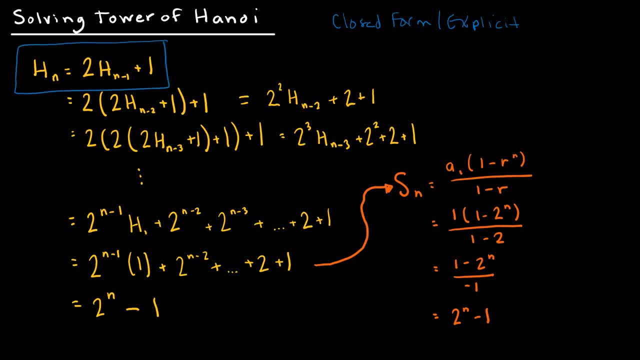 So this is the formula that we came up with previously. This was our recursive definition. To find the next value in the sequence, we take two times the value before it and then we add one, And if you'll notice, what I've done here is I've said: OK, well, what about this guy? 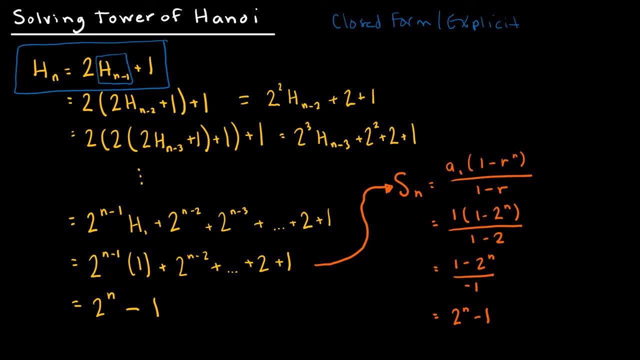 Can I do anything with that? This is that iterative approach that we've used previously in this course. So if I wanted to know what is h of n minus one? according to this definition, I would take two of h? n minus two plus one. 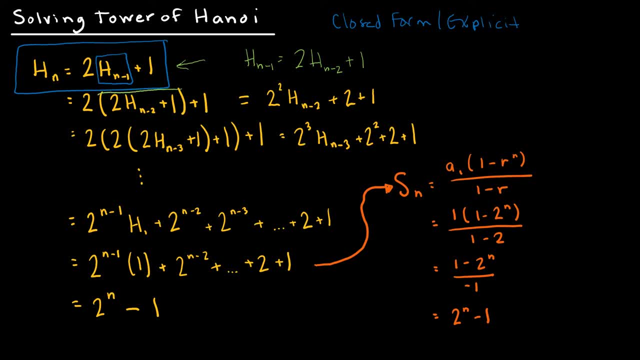 And so notice, I've just replaced that value for h n minus one, And then I did that again for h n minus two. I replaced it with two h n minus three plus one, And the reason that I'm doing that Is, of course, to try to find a pattern. 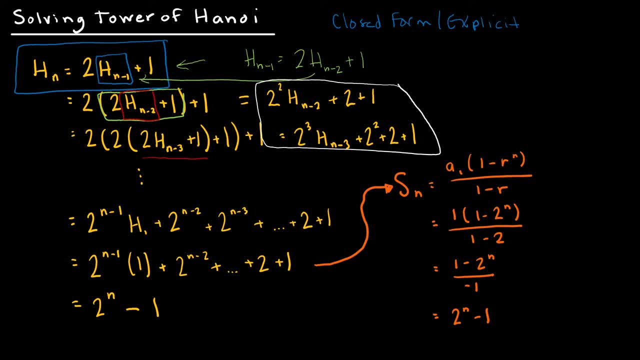 So this is the pattern that I'm starting to develop and I can see that I'm taking two to some value times the previous value And then notice I've got some more going on over here. So this is the definition, or this is the pattern that I'm starting to see is that I have two to the n minus one times h, one plus two to the n minus two. 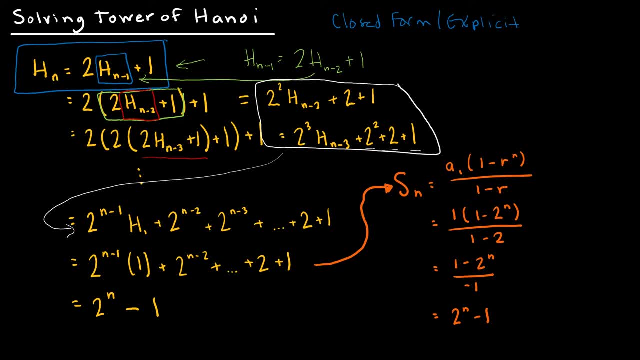 Plus Two to the n minus three, plus two to the n minus four, all the way up until I get to the n minus n minus one, which would be two to the first and then two to the n minus n, which is two to the zero or one. 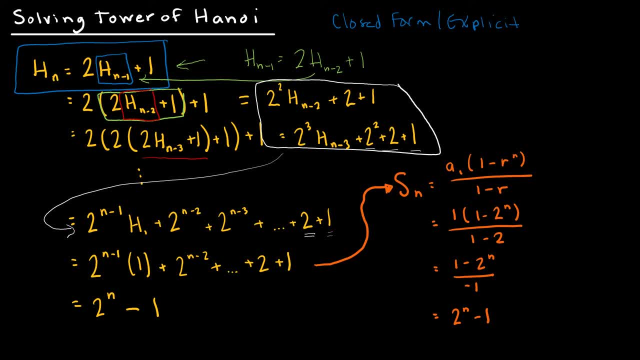 So I can see that that's the pattern that's happening And notice now all I'm going to do is replace this h one with the value for h one, which we determined in the other Just a moment ago, that it was just one move to take one disk and move it to the proper position. 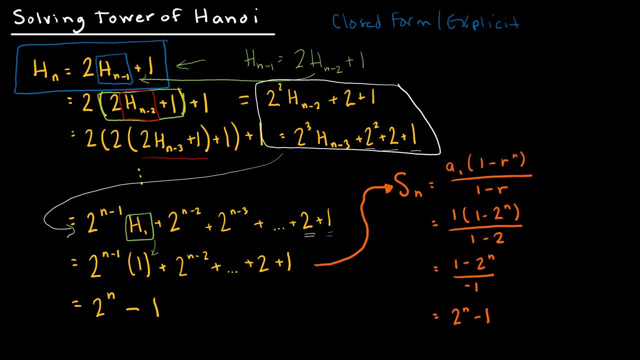 So I've replaced h one with one. So now what I'm looking at is that I have two to some power, and that power is continually decreasing. Well, what I know about a series like that or a sequence like that is that it's a geometric sequence. 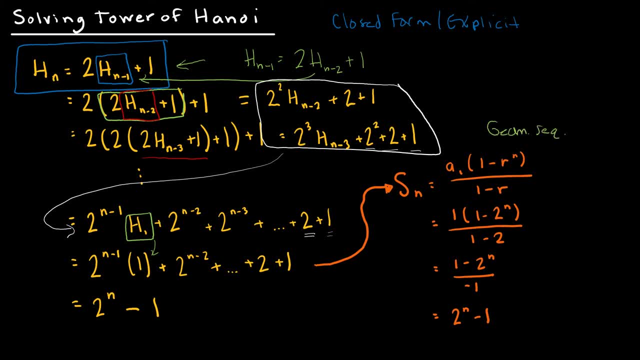 That's this, And I'm just going to use the formula for a geometric sequence to simplify all of this. And so what I'm going to do is I'm going to say: I know that I have an, a value and an r value in a geometric sequence. 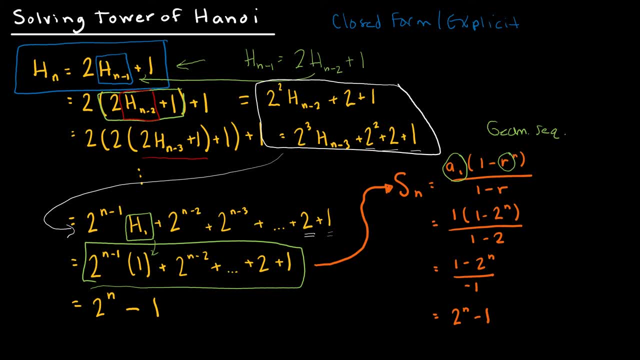 And the a value is some initial condition which we already determined was one, And the r value. is that common ratio or what it is that we do to get from one to the next? So to get from one To the next value, I would multiply by two, because of course that's what's happening here. 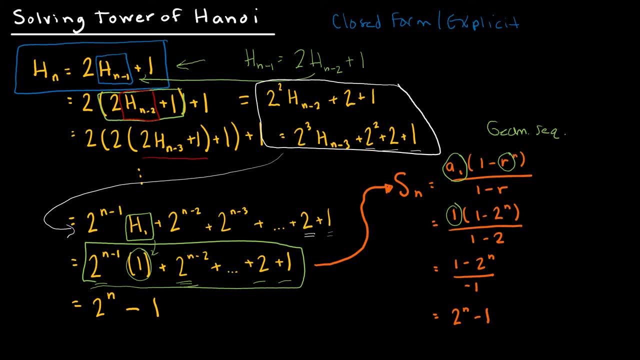 And to get from one to the next value, I'd multiply by two, And so that is my, are both here and here, And then I'm just doing some simplification, So I didn't didn't really care about the one, because when we multiply by one it's just one. 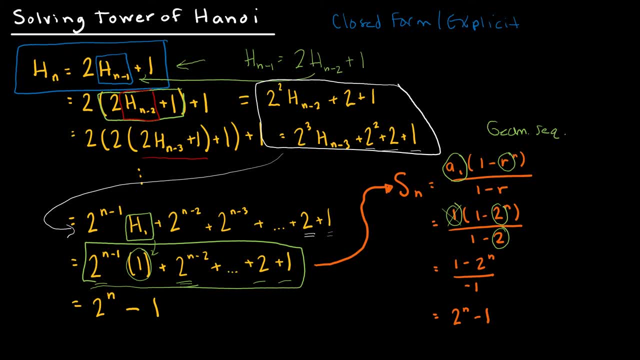 So, on the numerator, I have one minus two to the end, and my denominator, one minus two, is negative one. And then, of course, I just simplified that by distributing the negative one. And then, of course, I just simplified that by distributing the negative one. 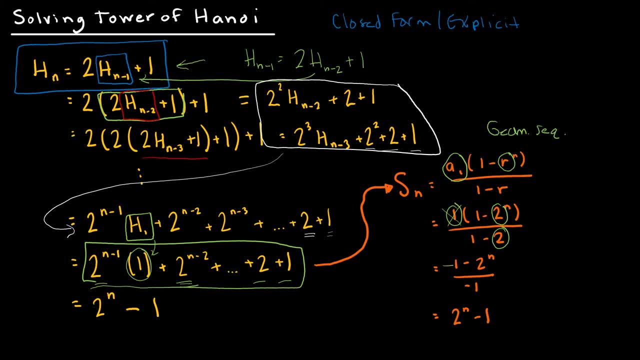 So I had a negative one and positive two And then I wrote it as two to the n minus one. So this is actually my closed form expression for solving the Tower of Hanoi. So if I wanted to know how many moves does it take to move five disks, I would take two to the fifth and subtract one. 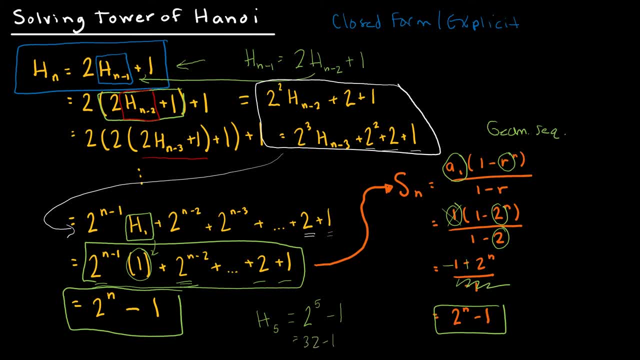 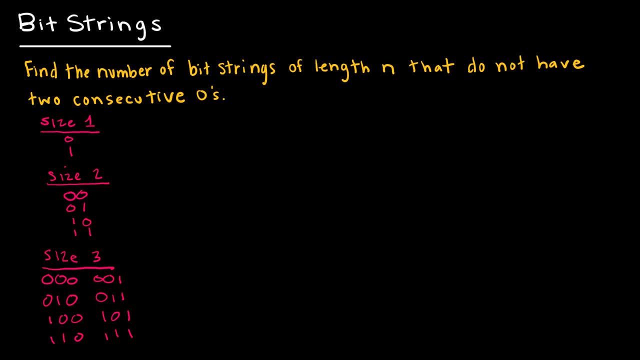 So two to the fifth is thirty. two minus one would be thirty one. So that's the total moves. Let's take a look now at a bit string question. We want to find the number of bit strings of length n that do not have two consecutive zeros. 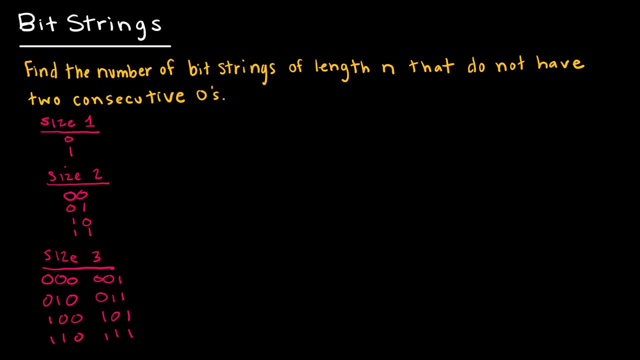 And there is an easy way to do this, which is just to find the answer, And then there's, of course, the harder way, which is to understand why the answer is the way it is. So I would challenge you to be that second student that tries to understand why the value is the way it is, so that you can apply that knowledge to other questions. 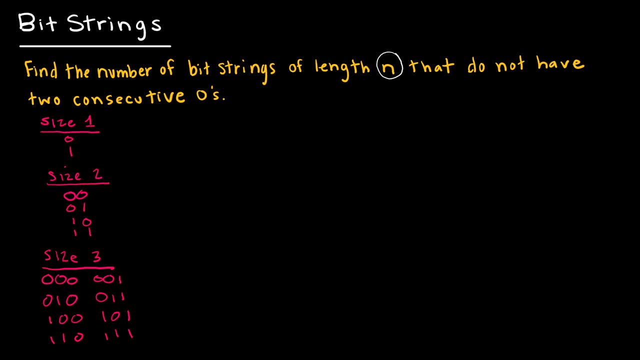 We here are looking for the number of bits. strings of length n. We're looking for length n bit strings that do not have two consecutive zeros And, if you'll notice, I've written out size one, size two and size three already, but I haven't taken into account that I don't want two consecutive zeros. 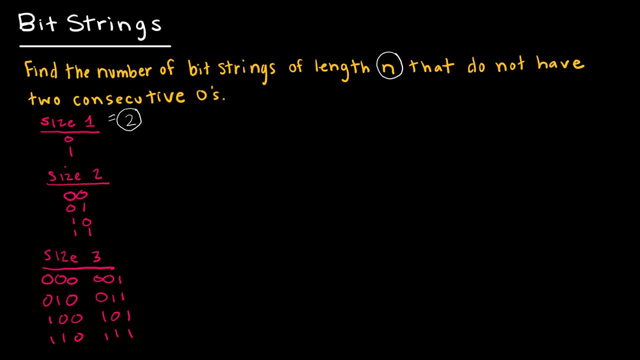 For size one, both of my answers work, because it's obviously size one, So I can't have two consecutive zeros. for size two, The only value that doesn't work is the double bit string of zero- zero. So there are three here, and then for size three. 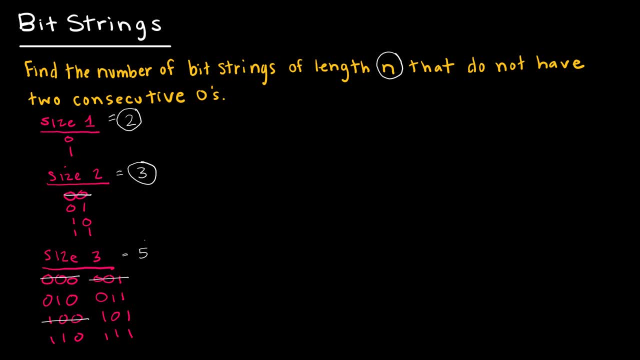 I have to get rid of three of them, And so there are five total that don't have consecutive zeros. So the easy way out is to say: well, two plus three is five, So maybe that works, And then you would find size four. 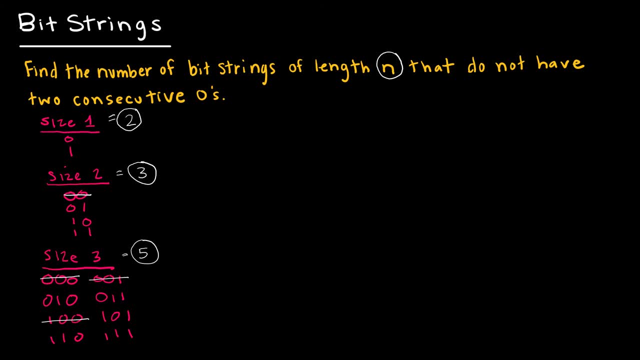 And if size four had eight possibilities, then you would feel pretty confident in your abilities to say, just add the two values before. But let's make sure we understand, or verify, that that in fact works. So what I want to do is I'm going to write. 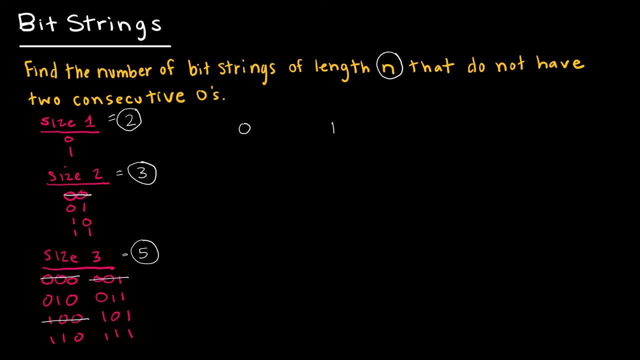 The two of size one that I have and the three Whoops. I'm going to do it this way: One zero And one one and zero one, And I'm going to try to sort of match those up to what I have in size three. 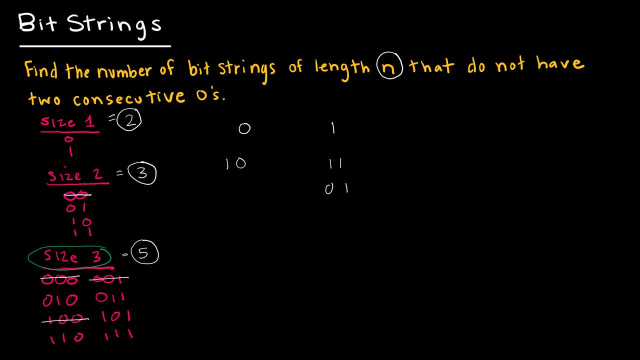 So I have one zero, or sorry, zero, one zero. This guy right here. I'm going to add a one zero to the end of zero. And then I have One zero And I'm going to add a one to that, one zero one. 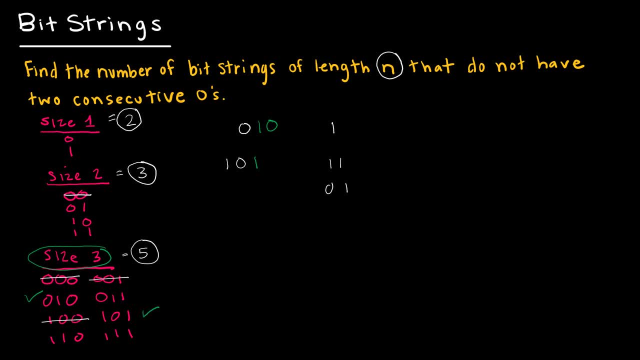 So I've used that one And for one, Sorry, for one one I've got one one, one, One, one one. And for zero one I have zero one one, And for the last one I have one one, zero. So my question is: do you notice any pattern with how I've done this? 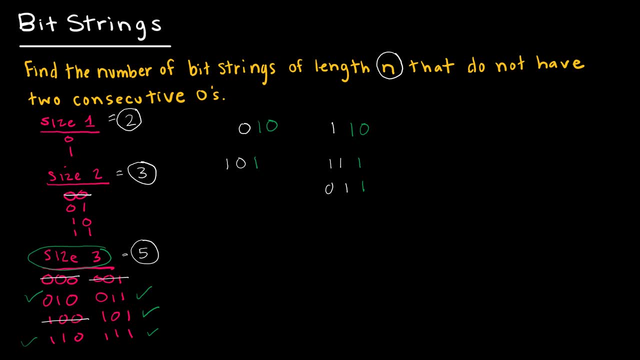 How did I go from size one to size three and from size two to size three? Because that's sort of our conjecture. It's That we would just add two plus three. But why does that work? Well, let's take a look at the size ones. 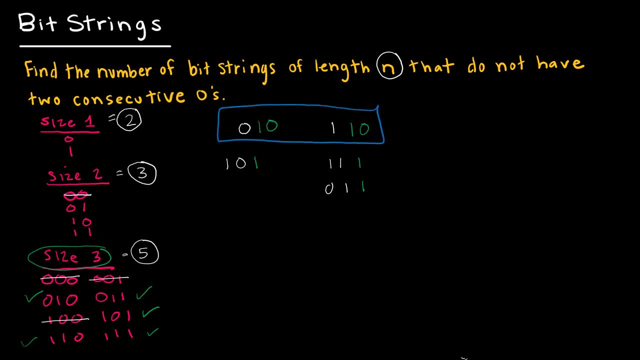 For size one. It looks like if it was size one, I added a one zero to the end of it, And if it was a size two, I added a one to the end of it. Now does that make sense? Could I continue that pattern? 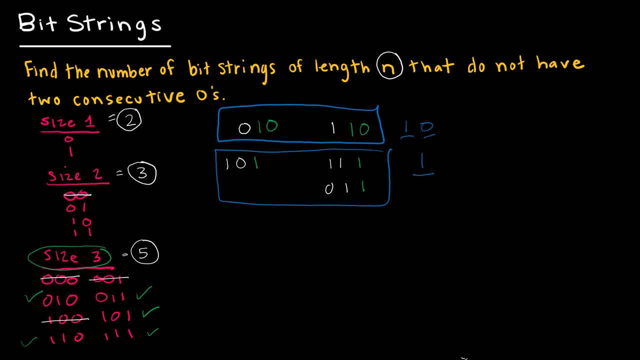 Well, it does make sense, because what I'm basically saying is, if I have a total of n bit strings, if this guy is a one, then it doesn't matter what the value is right before it. It could be a zero, because zero one doesn't break any rules of having two zeros in a row. 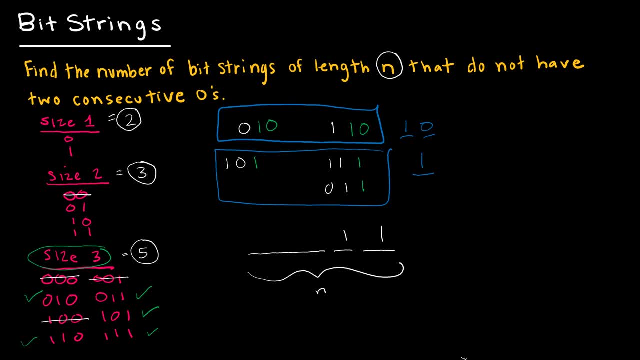 or it could be a one, Because having two ones in a row doesn't break any rules. So all of these values before my last value is n minus one values. So I'm taking that and then just adding a one to the end, And then for my other situation where I have two values,